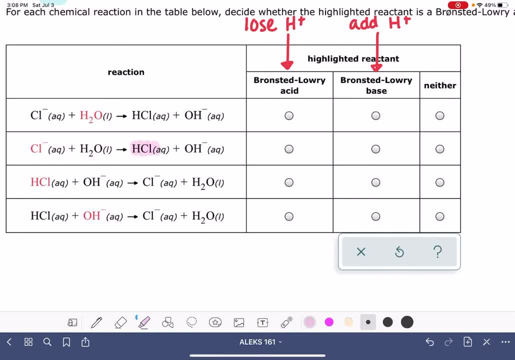 conclusion that the chloride becomes HCl. We can link those two together and once you've made that determination that those two- this reactant- belongs with this product, then you can apply these definitions of the Bronsted-Lowry acid and base. What happened to the chloride in terms of 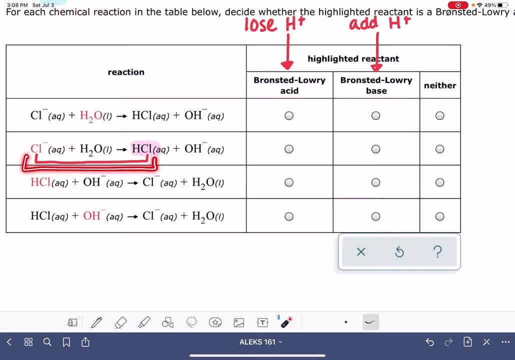 the definitions of acids and bases. We can see that the chloride ion added a hydrogen ion, which is the definition of what it means to be a Bronsted base. So we'll check that box. It's easy to see that it added the hydrogen atom because it went from Cl to HCl. It's not quite as easy to see. 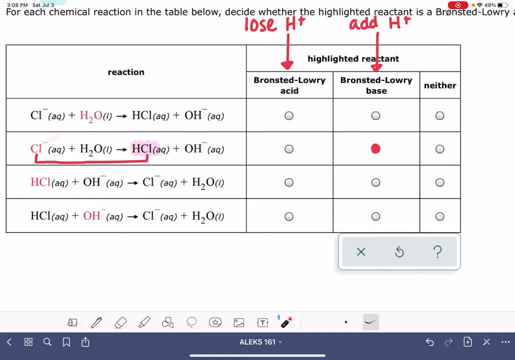 that it added the positive charge. but if you think about it, it started as a negative charge and then we added a positive charge And it ended up as a neutral molecule over here. So, like I said, the first one is a little bit. 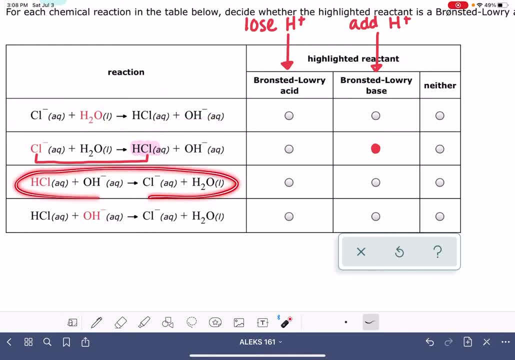 trickier to visualize. So what I'm going to do is like skip on down to the next one, because this one's going to be a little bit easier as well. We're focusing this time on HCl, because it's red. So what we want to do is think about, for our two products, what did HCl turn into? Use your common. 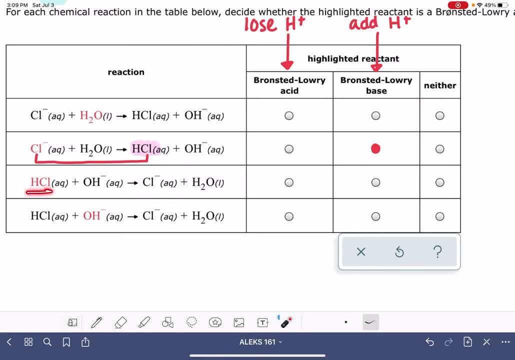 sense. Use your, just your- good chemical intuition. HCl is going to turn itself into the molecule that most closely resembles HCl. So we want to pick. when we're looking for what did it turn into? We want to pick the product that most closely resembles HCl in terms of atoms, like what atoms are present? 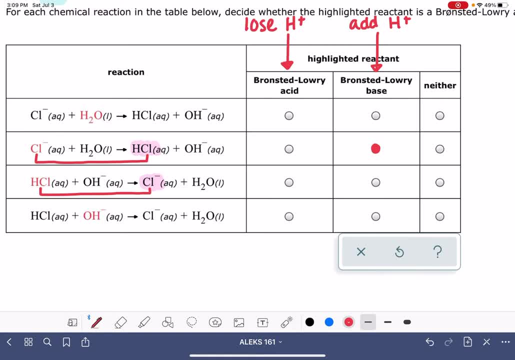 Once we have made that decision, we know that we can pair up the HCl with the Cl minus, and then we can analyze: how did this transformation take place? What happened to HCl as it turned into Cl minus in the context of the Bronsted-Lowry acid definitions? 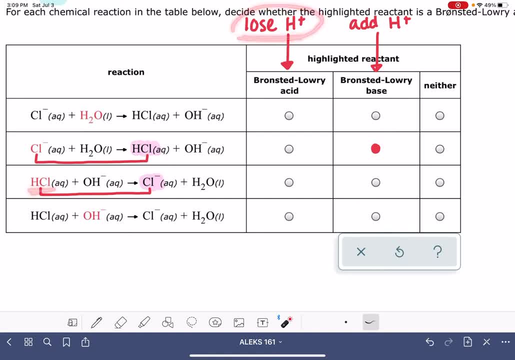 It has HCl, has lost an H plus, which makes it an acid right there. Okay, so let's move on down. Let's actually let's just go ahead and go back up to the harder one, this harder one up on the top. 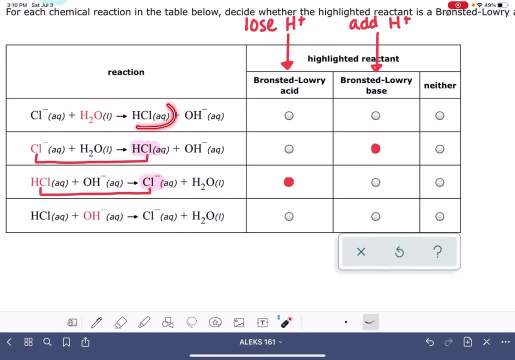 So we're focusing on H2O and we want to ask ourselves: what did the H2O turn into? And this one's a little bit trickier to see because the atoms get rearranged in the way that we conventionally write these different molecules.